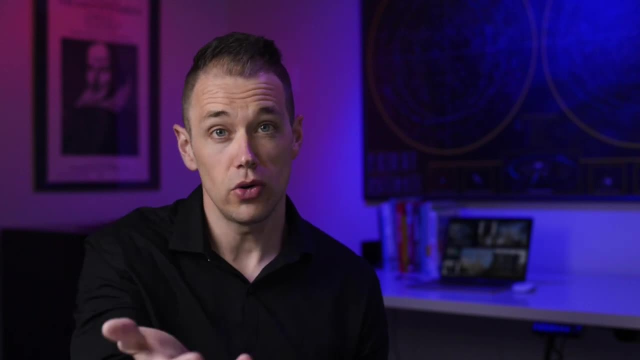 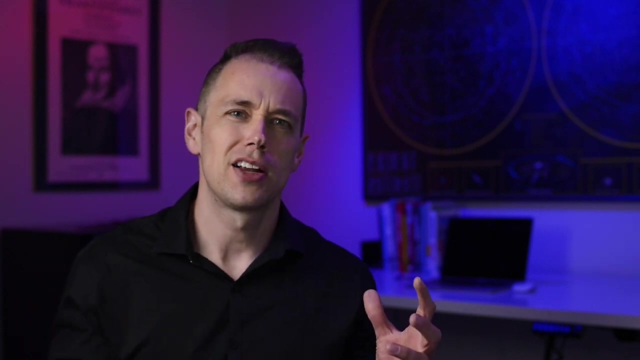 industry And the other is how many users could become your users, that is, find value in your app. In a previous video, we came up with an app concept that was kind of like matchcom meets your dentist's office. It's kind of like a social marketplace where dental office managers can. 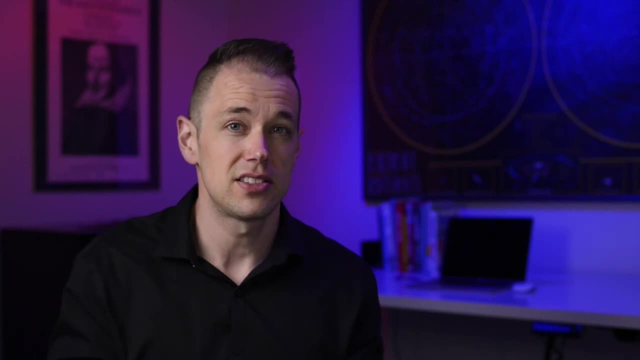 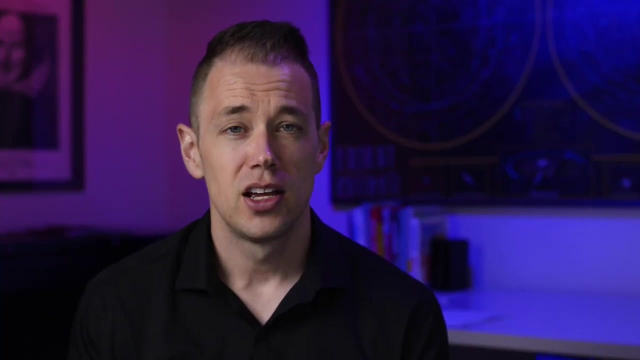 go and find candidates to hire as dental assistants or dental office administrators, So we're going to use that as an example For this video. finding market size data really is not hard. The reason why is because there are market research firms that want to sell their market reports to you, And in order to do that, 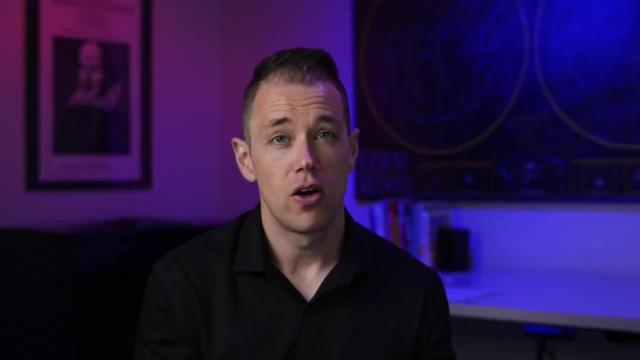 they usually give you a sample of their data. All you really need are the headlines from the promotional materials for these market reports. You don't need to buy the whole report. You just go and look and you say, oh, this is the market size for this industry for this year. 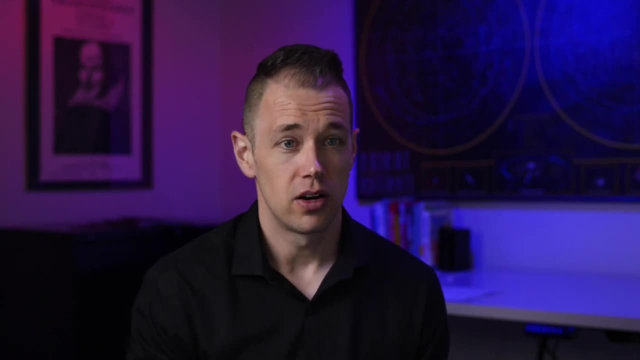 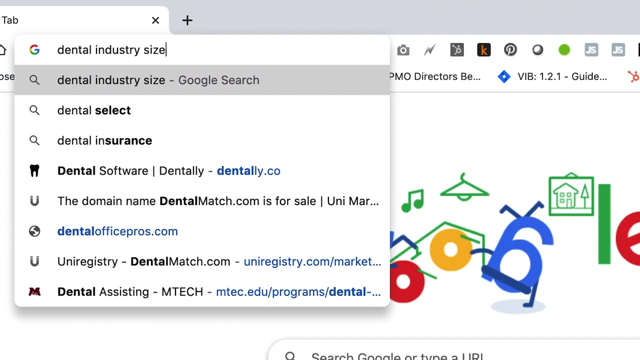 So one of the easiest ways to do that is to just do an internet search for name of industry, then industry size. So I'm just going to do a simple search for dental industry size And voila, this report from IBISWorld comes up: dentists in the US market size And it tells me: 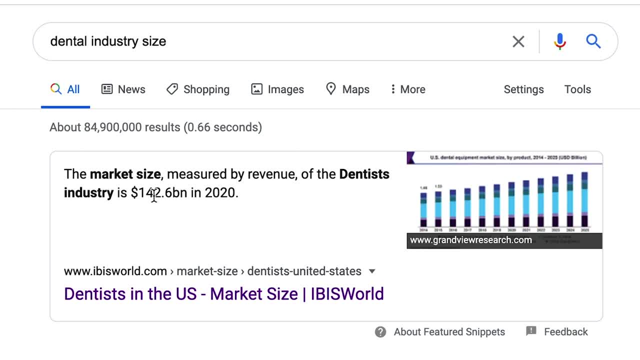 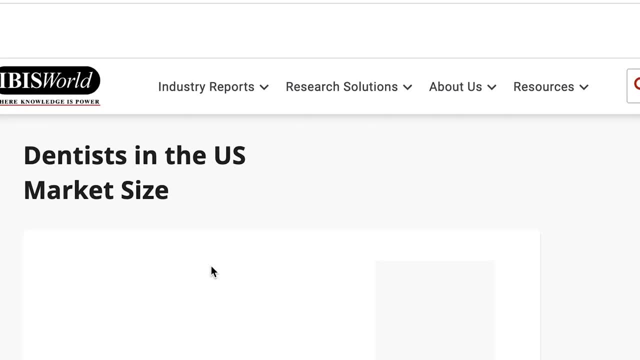 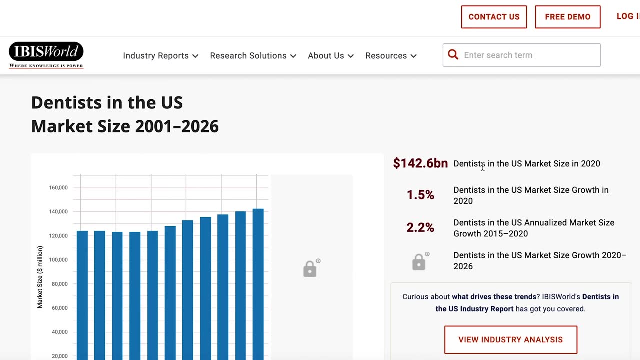 the headline right here in the Google search results. The market size, measured by revenue, of the dentists industry is $142.6 billion in 2020.. If I click on this, I go over to the actual report itself And it shows me again one hundred and forty two point six billion dollars: dentists. 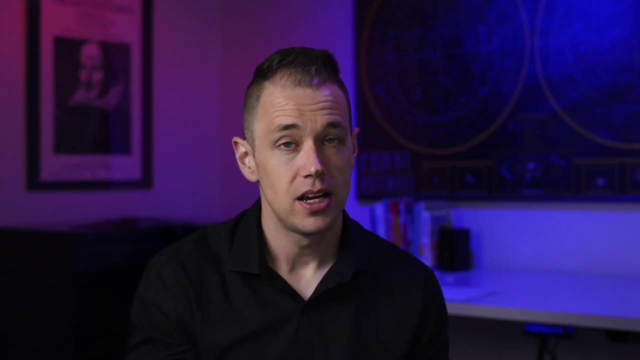 in 2020.. And it's increasing. This is how much money is channeling through the dental industry in the United States, And that's not the only statistic that we're concerned about. We want to know how many users we're going to have. And, in the app concept, 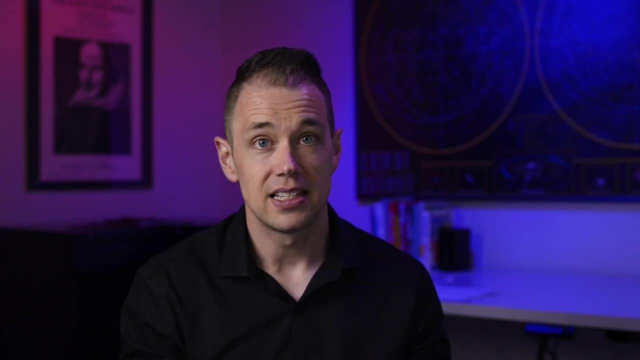 we said that the user persona. there are actually two of them: One is the dental office manager and the other are all the candidates that want dental office jobs, So the office admin or the dental assistant. So let's assume that there is one dental office man. 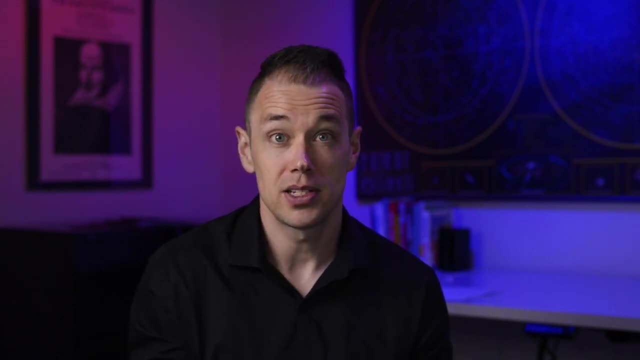 and there's a manager in every dental office. That's reasonable, At least one. Maybe some have more than one, but we're going to assume that every practice out there has someone who is not a dentist managing everything else: Paperwork, insurance, billing, appointments. 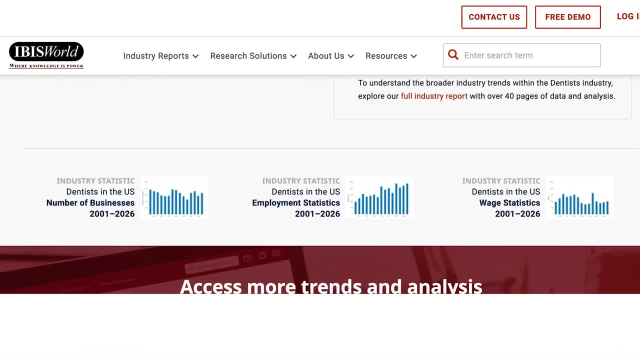 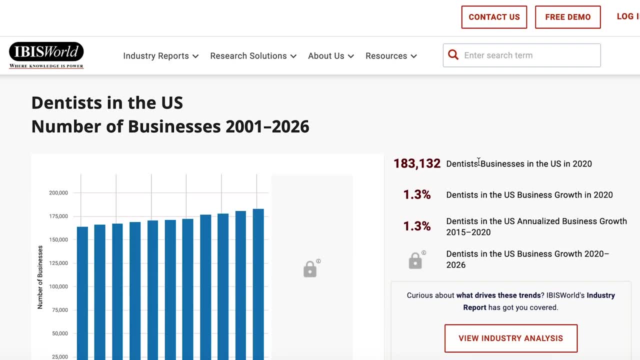 all that stuff. So let's see if anything else here in this report can be useful. If I scroll down I can see aha, dentists in the US. the number of businesses- jackpot. So looking at this report it says, hey, there are one hundred and eighty three thousand one hundred thirty two dentist. 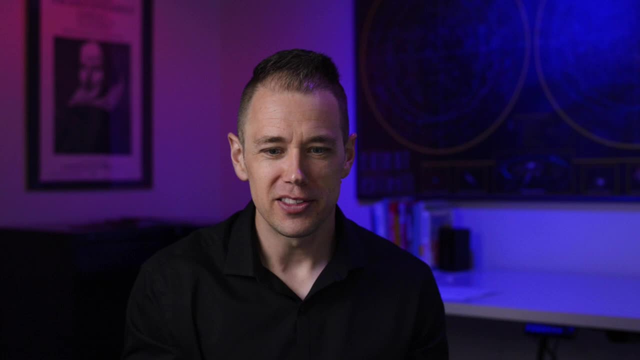 in the US in 2020.. So we can assume, then, that there are one hundred and eighty three thousand one hundred and thirty two or more dental office managers out there waiting to use our application, But that's only one user persona. We still had another persona. that was the job seeker. 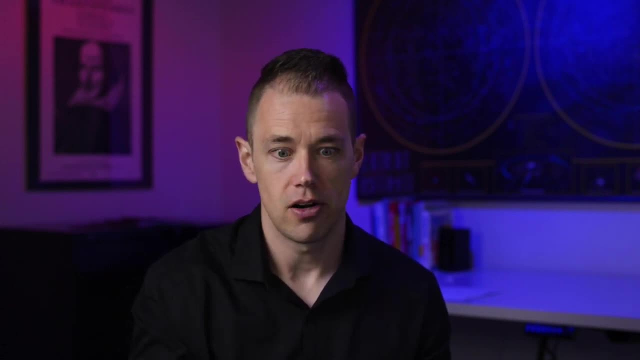 right, The candidate. How can we figure out how many of those users there are? Well, if we know how many businesses there are, that gives us the perspective on how many office managers there might be. But what if we could find some kind of an employee report that would tell us how many employees there might be. Well, if we know how many businesses there are, that gives us the perspective on how many office managers there might be. But what if we could find some kind of an employee report that would tell us how many employees there are in the dental industry? 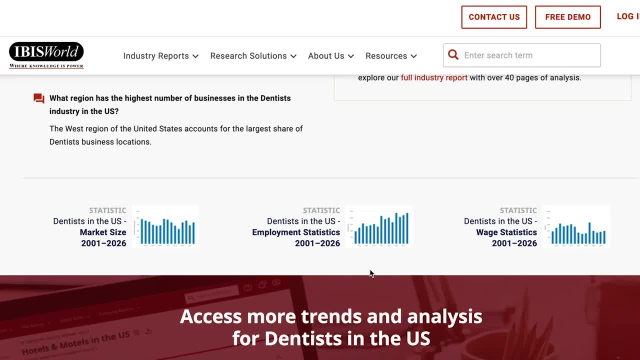 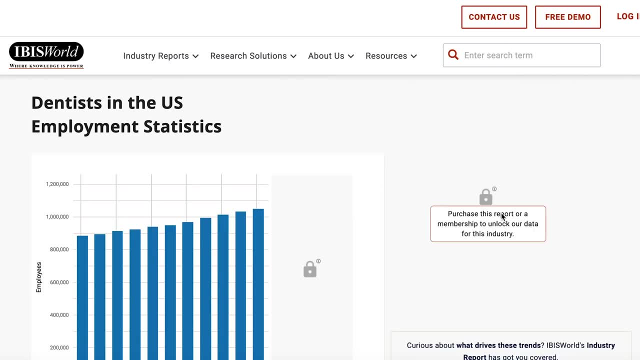 in the US. So let's look at that. Aha, It's right here: Dentists in the US- employment statistics. So if I go and I view that report, see right here it's telling me that this report is locked, because I actually already viewed this page yesterday, So it's probably counting the number. 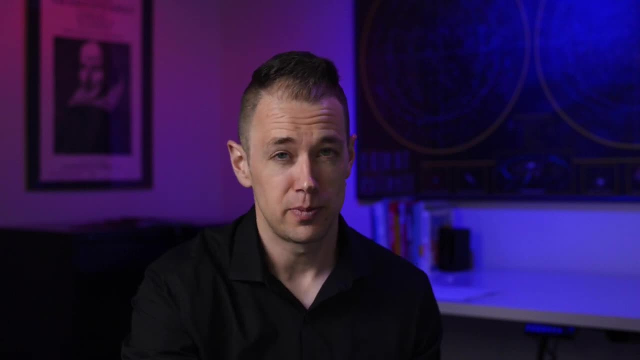 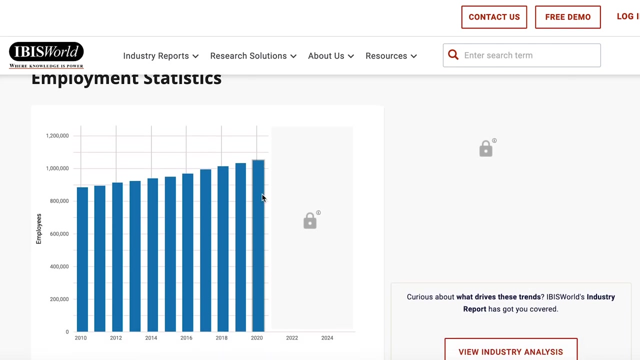 of times I visited their website. I already know the number because I saw this page yesterday. But let's check one thing. over here There's this bar chart with some live data on it. What happens if I click here? Aha, So. it shows me, in 2020, there were 1,049,889 dental employees. It took us about five minutes to find the market size and the number of users for this application. Now I know there are 183,132 dental businesses in the US. We can assume that each one of those offices has a dental office manager. But not everyone is going to use this app. Even if we were to just take 1- 20th of that number, that means there are 9,156 dental offices in the US. That means there are 9,156 offices in the US. That means there are 9,156 office manager users that could get on our app. I also know that there are 1,049,889 dental employees in the US. Even just a 20th of those people would be 52,494 candidate users in our application. So assessing market size: not hard, not long. 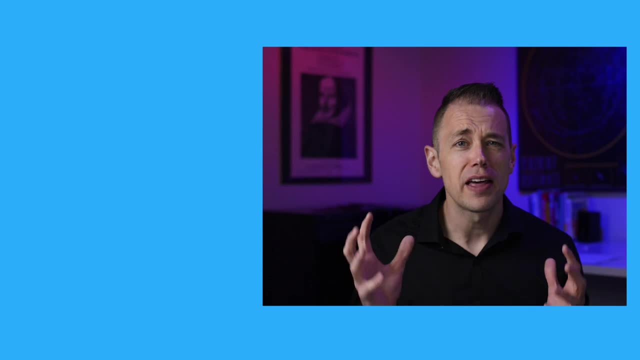 Coming up next on Build Your SaaS. Out of all of the app ideas out there, all of the genius business models you could possibly think of, how do you know which one of them is the best? Let me know in the comments below And I'll see you in the next video. 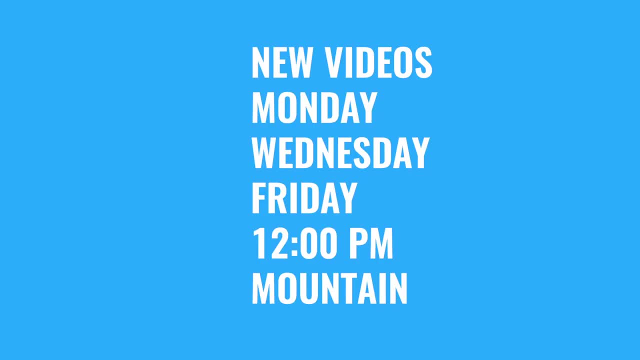 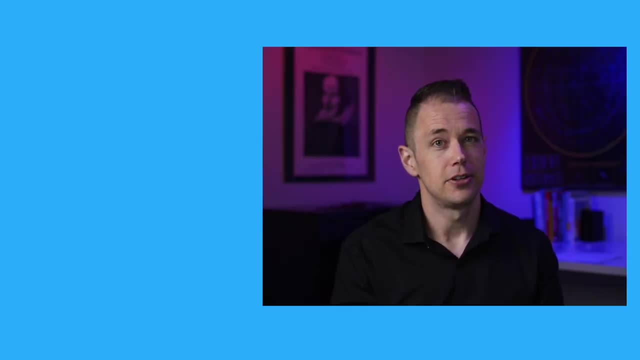 If you like this little video, give a like. If you like this little video, hit the like. If you want to join our tribe, then please hit subscribe, Hit the bell and give this video a like.